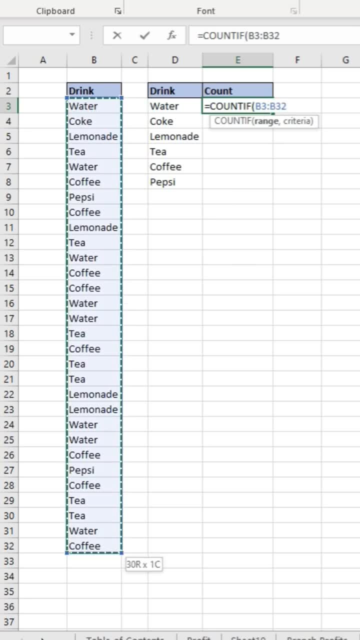 So use the count if function and then select our range And we're going to make this a absolute reference. So highlight it and press F4.. Then we're going to give it a criteria and say: count it if it's water, Close that and you're done. 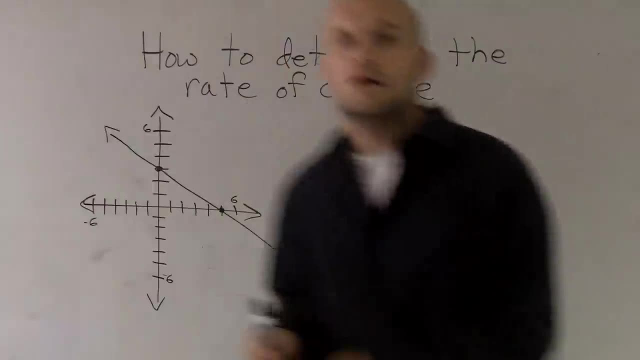 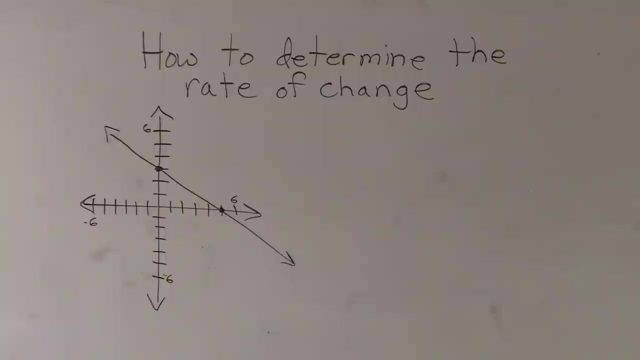 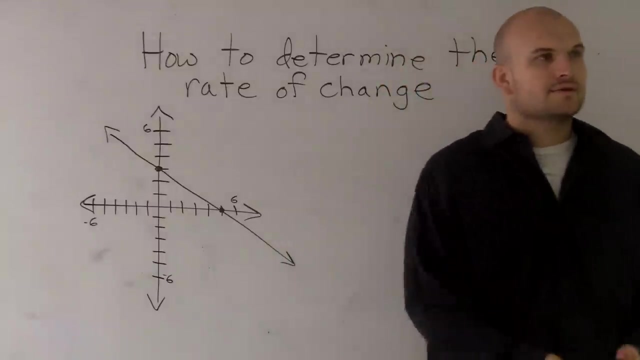 Alright, what I'd like to show you guys how to do is how to determine the rate of change when you're given a graph and when you're given when you can find two points from that graph. So, on this problem, right here I have a graph and I have two x and y intercepts. 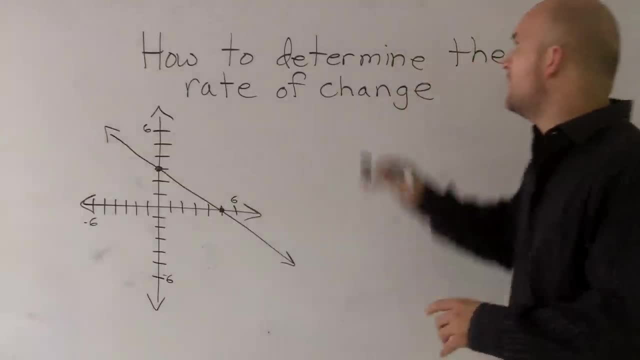 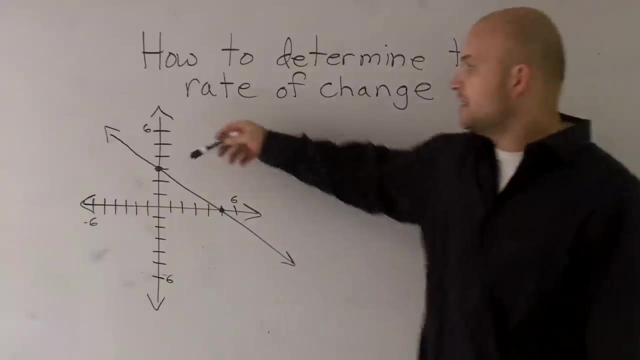 So I'm able to easily determine. those are going to be my two points. So when I want to determine the rate of change- remember the rate of change is the same thing as your slope- What we want to do is we want to see what is the change in your x variables and 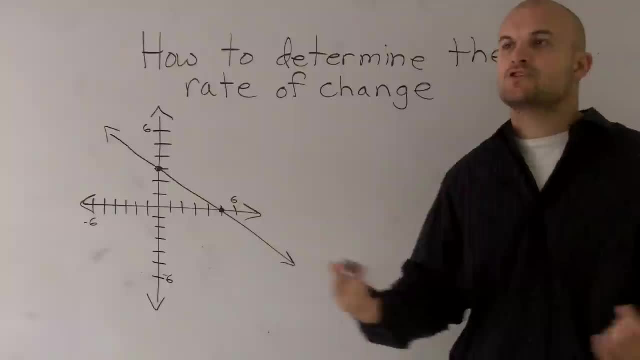 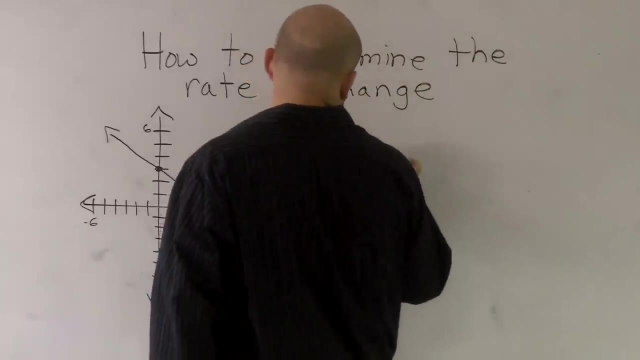 the change in your y variables. So there's a lot of different ways we can go and look or approach this problem. The first way is we're going to say, alright, well, if I want to look at, remember, let me actually write this down. So we have slope is the same thing.